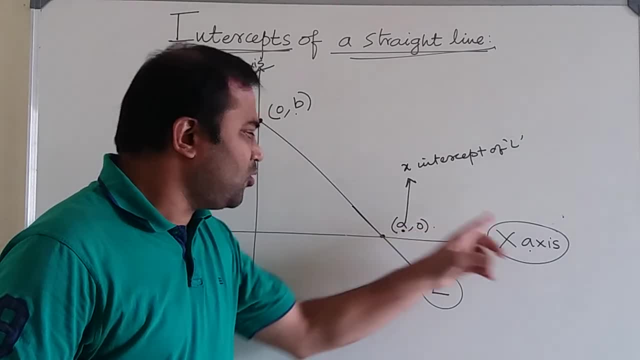 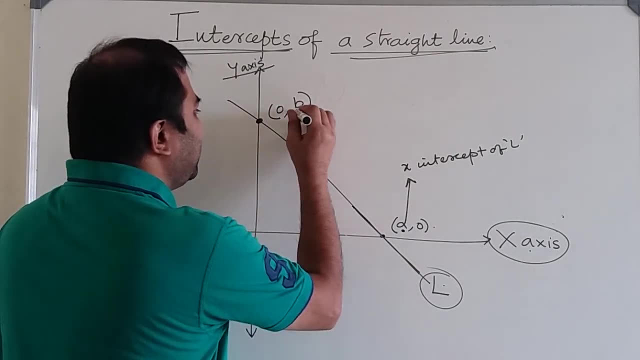 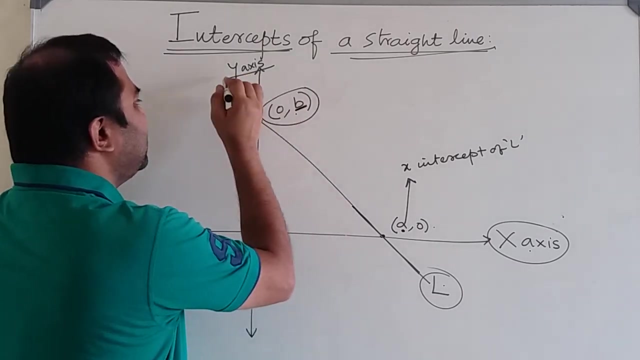 x-coordinate in the point A0, which is lying on x-axis And through which point the line is passing. Similarly, y-intercept of the straight line L is defined as the y-coordinate in this point lying on y-axis, through which the line is passing. 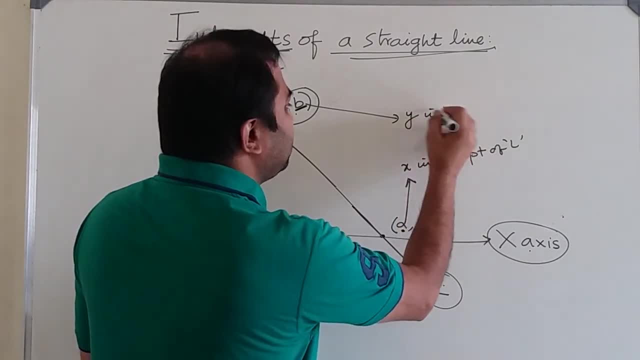 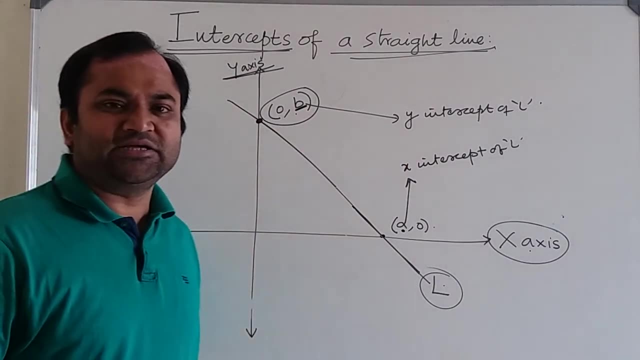 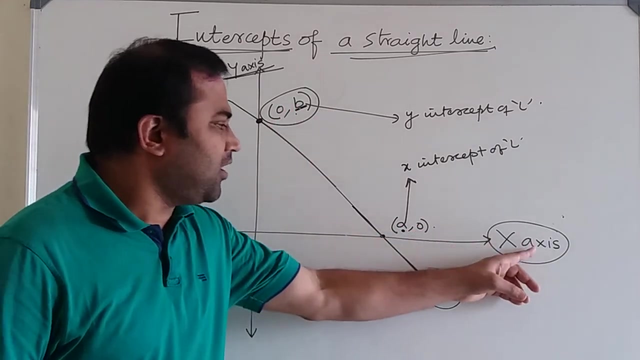 So B, the y-coordinate B is said to be the y-intercept of the straight line L. So x-intercept and y-intercept mean the x-coordinate And y-coordinate, in one word, In the respective points of the respective axis through which the line is passing. 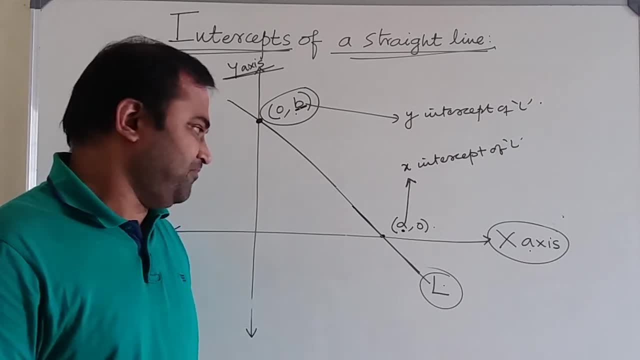 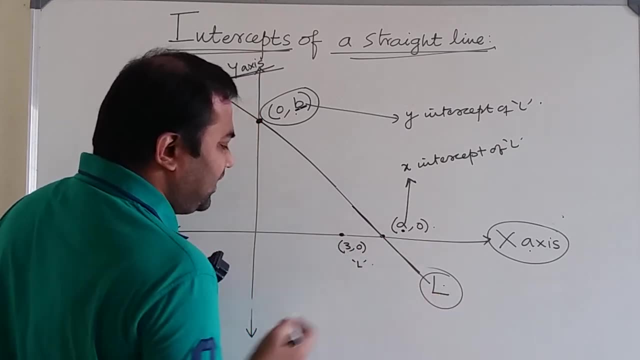 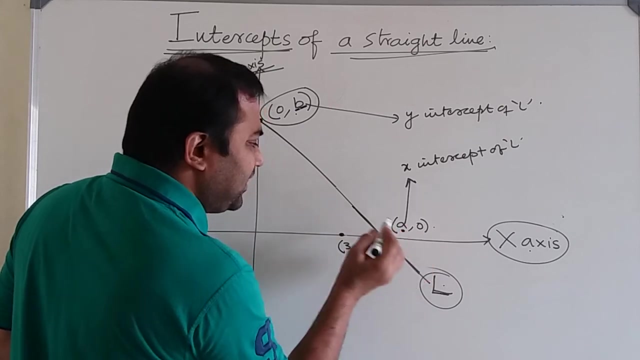 Intercepts exist with respect to a straight line. You cannot consider this point 3, 0 as x-intercept of the line L, Because you do not see the line L passing through this point. So x-intercept means the x-coordinate in the point. 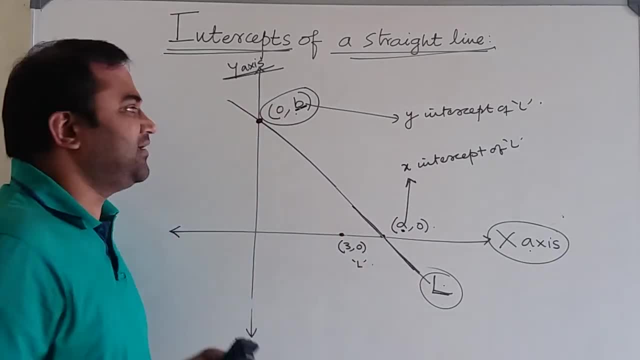 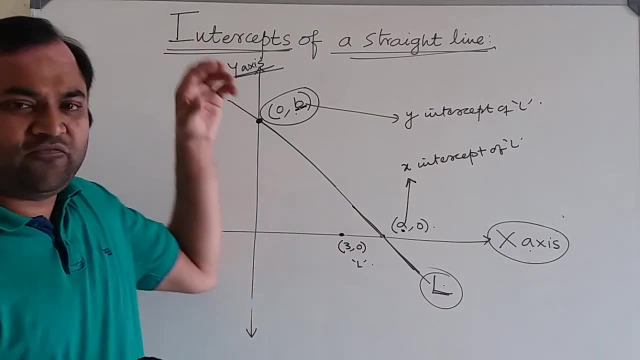 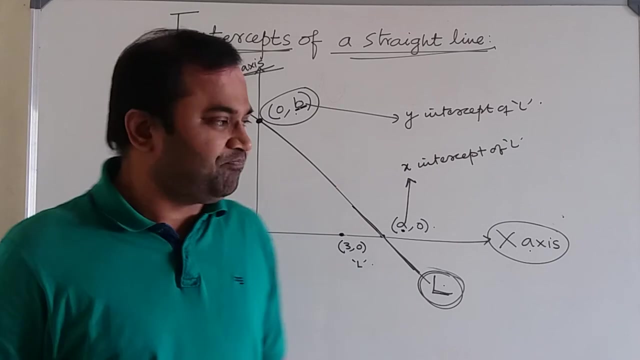 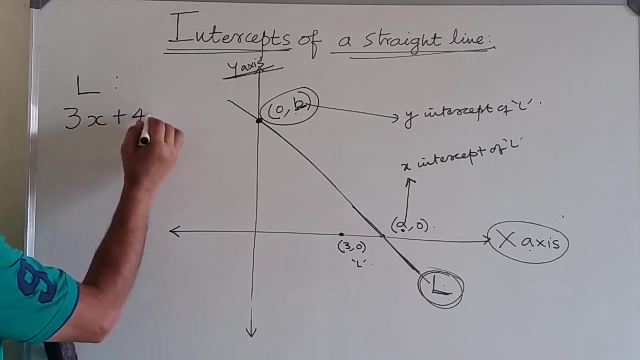 On the x-axis through which the line has to pass, Similarly the y-intercept. Now, coming to the next topic in this video, How to find x-intercept and y-intercept of a line L whose equation is given. Let me consider the equation of the straight line L to be: 3x plus 4y is equal to 12.. 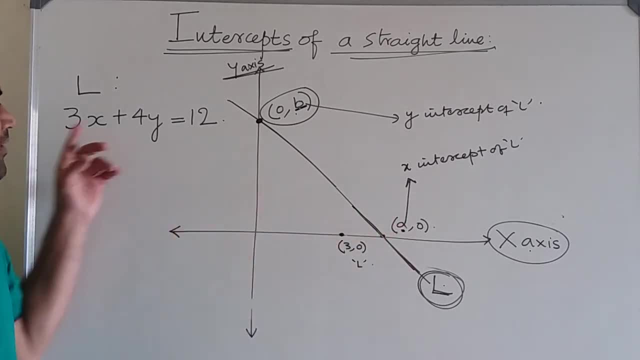 If we are asked to find the x-intercept of the straight line L to be: 3x plus 4y is equal to 12.. If we are asked to find the x-intercept and y-intercept of the straight line L, whose equation is given: 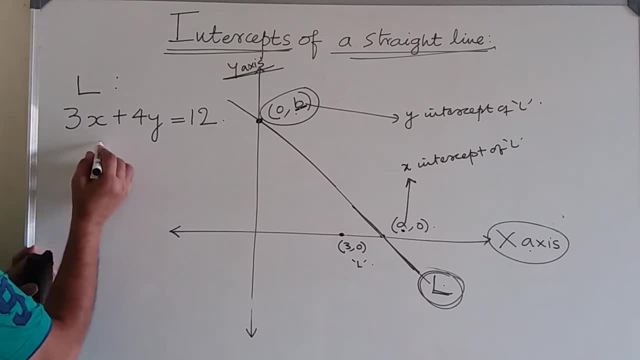 Then how do we determine It is this way? x-intercept means- you must remember it- as the point a0 on the x-axis through which the line is passing Now, since the point lies on the line, Therefore, you can substitute x-coordinate a in the place of x. 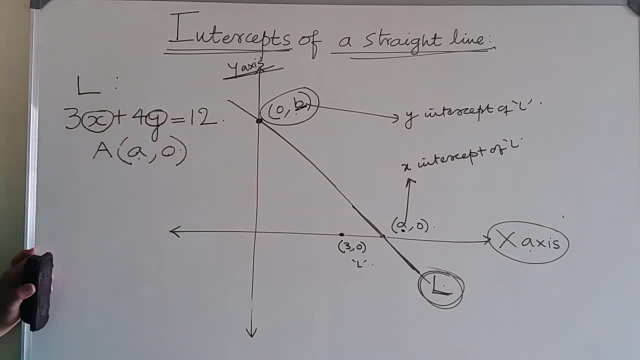 And 0 in the place of y and obtain the x-intercept. Let us do it: Substitute a in x, 0 in y, So that x-intercept a of this line L will be 4.. Similarly, determine the y-intercept.